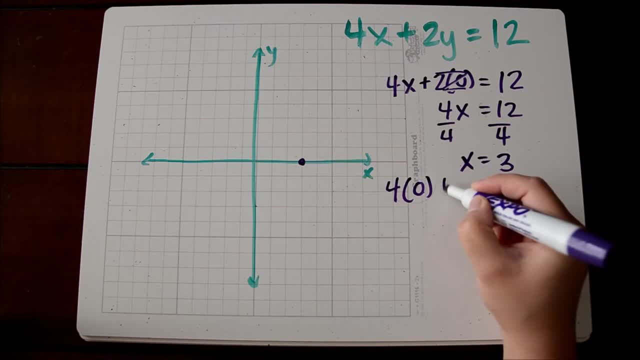 0 in for x, and so we get 4 times 0 plus 2x equals 12.. Anything times 0 is 0. We're left with 2y is equal to 12.. So we're left with 1 times 2y is equal to x, And we've added: 2 through x And we find that the y-intercept or the x-intercept, a basis, always comes from our x-intercept. So we have a prime-і which we know stands for the negative 2λ. then it's the result that we find the x interval, We get 1y and weapon, But Because again we have line sandwich. 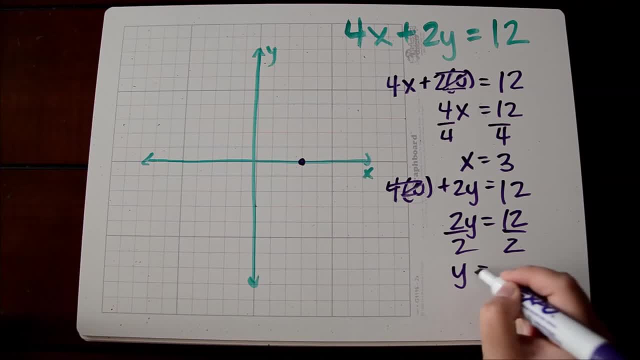 and when we divide both sides by 2, we get y is equal to 6. And so that means we have a y intercept at 0, 6, because our x value is 0. And so using these two intercepts we could go ahead. 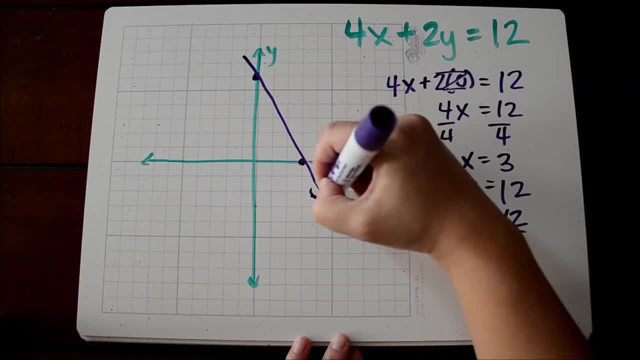 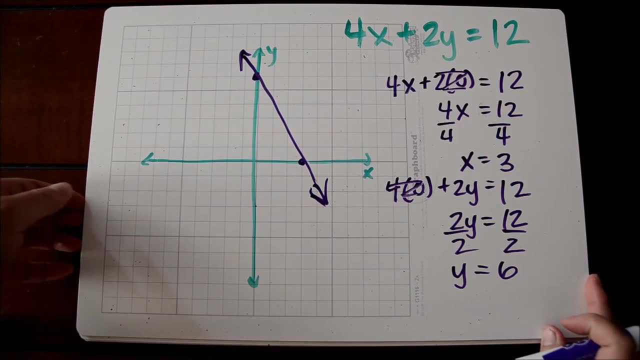 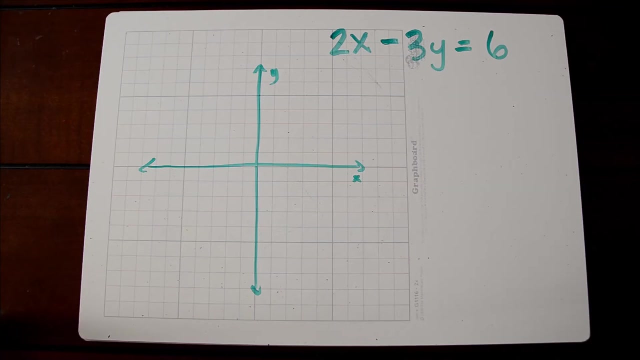 and connect them with a line, and that is how we would graph this equation. that's written in standard form. Let's take a look at another example. So here we have another example of a standard form equation. We're first going to find our x intercept by substituting in 0 for our y. 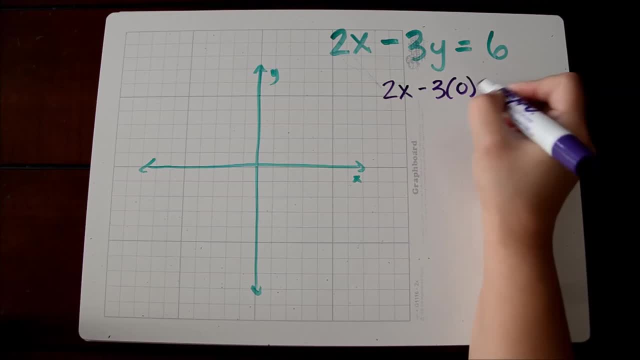 and so we get 2x minus 3 times 0 equals 6.. Anything times 0 is 0, and so we're left with 2x is equal to 6, and when we divide to solve for x, we get x is equal to 3.. 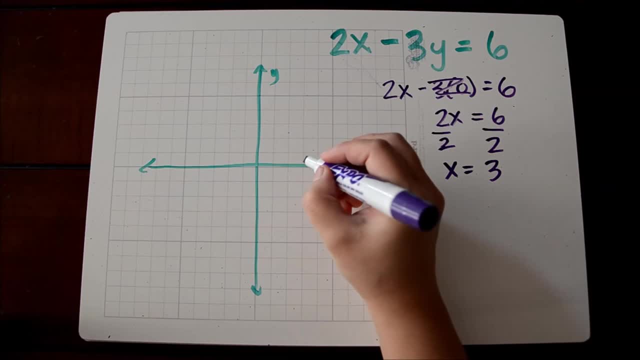 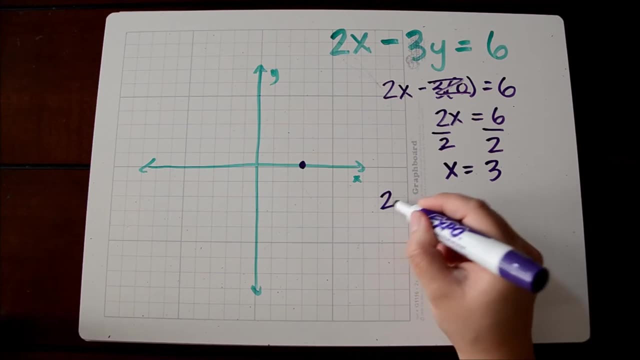 So that means our x intercept is at 3, 0 because the y value was 0. And now to find our y intercept, we're going to substitute in 0 for x, And again, anything times 0 is 0. so this is gone. 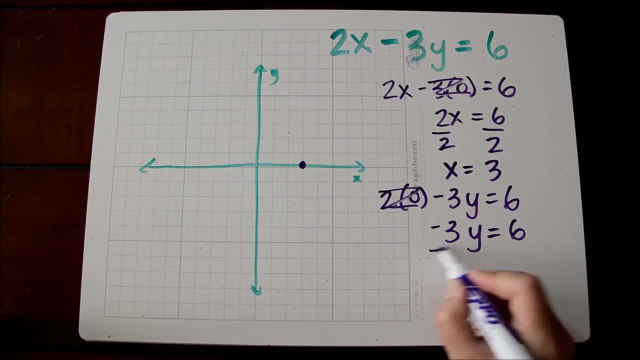 We're left with negative. 3y is equal to 6 and when we divide both sides to solve for y, we get y is equal to negative 2.. So we're going to have our y is equal to negative 2 and we're going to have our y is equal to negative 2.. 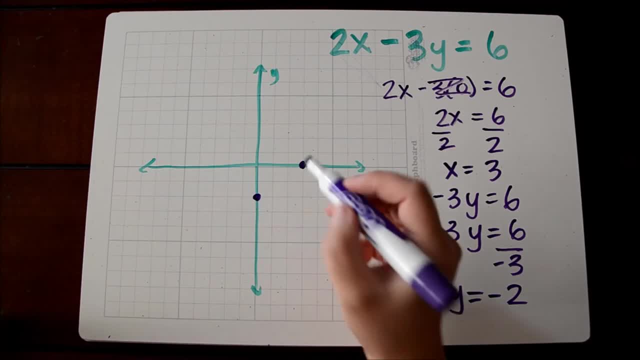 So we're going to have our y is equal to negative 2 and we're going to have our y is equal to negative 2.. So we're going to have our y is equal to negative 2 and we're going to have our y is equal to negative 2.. 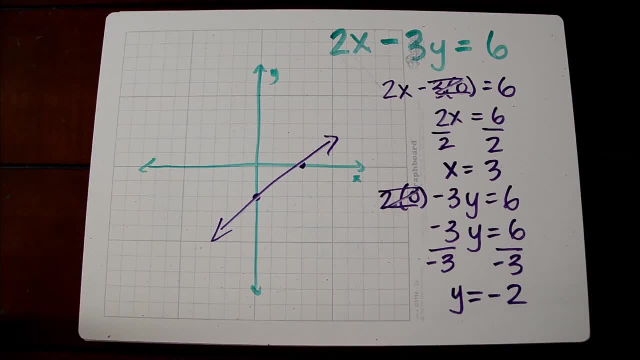 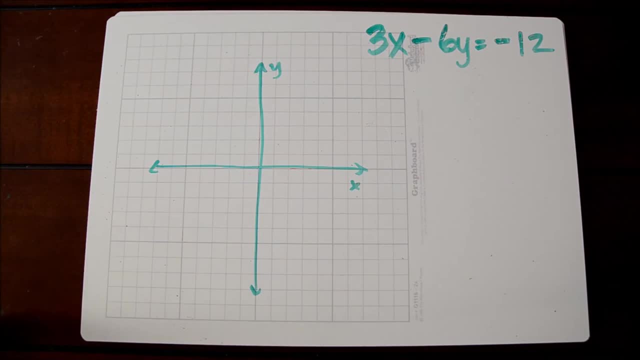 And when we connect our two intercepts. this is the graph of our linear equation. Let's take a look at one more example. So again we have an equation written in standard form. We're first going to find our x intercept by substituting in 0 for y.